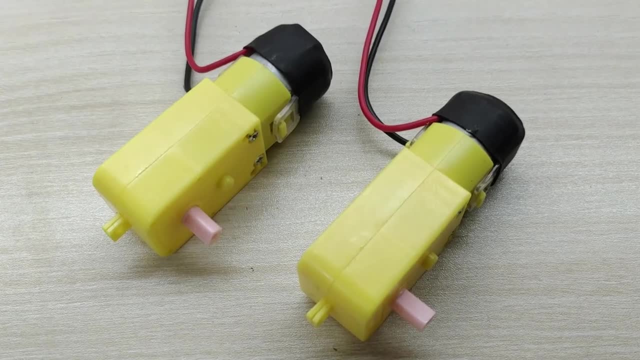 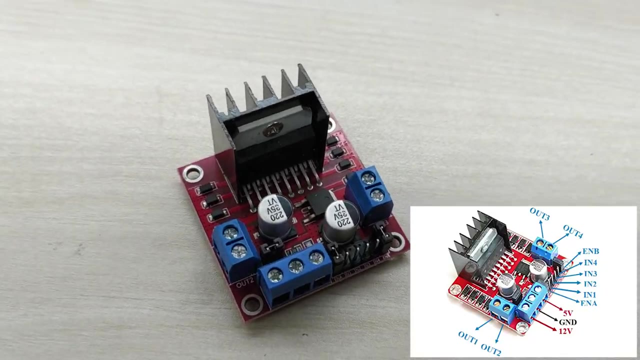 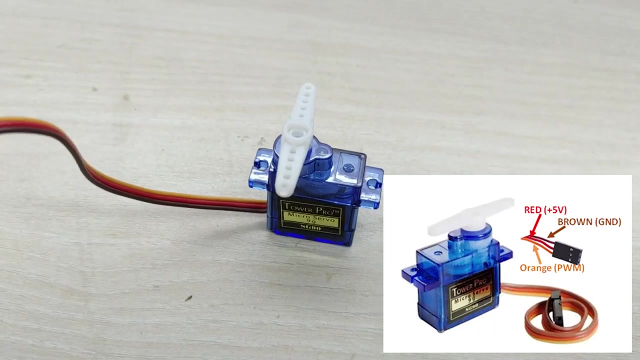 For this project you need two numbers of geared motors, two numbers of 65mm diameter wheels, Arduino, Uniboard L290A10 motor driver module, HCSRO4 ultrasonic sensor, SG90 servo motor and a caster wheel as the main components. 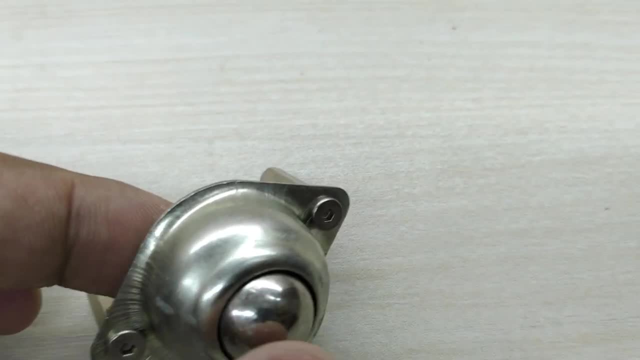 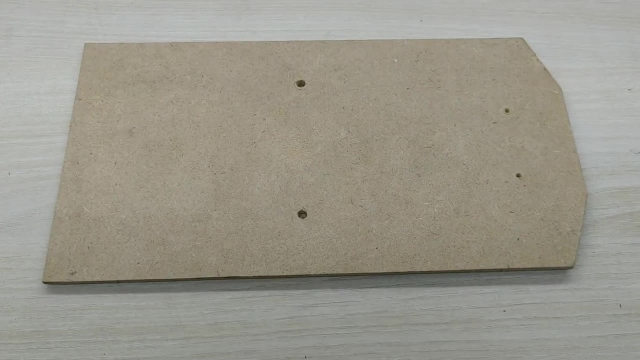 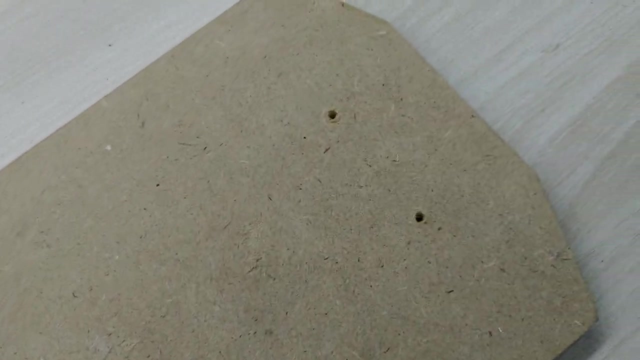 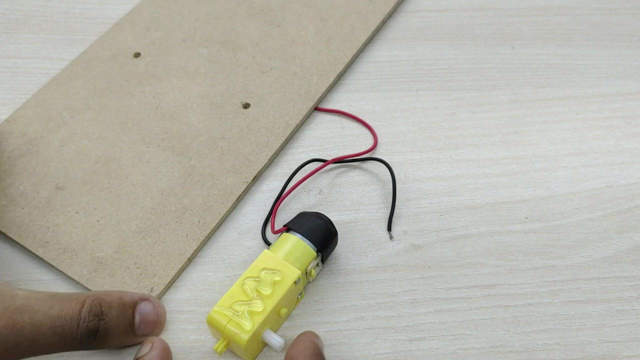 The caster wheel has a ball inside it which can roll in any direction. First take a plywood board and cut into the shape as shown. Also make two holes for the motor wires to pass through and also for fixing the caster wheel. The drawing template for the plywood is given in the description box. 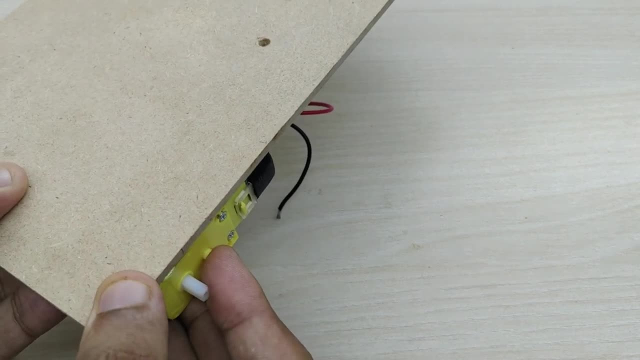 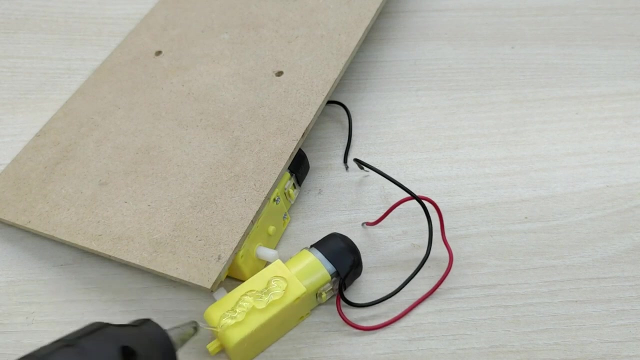 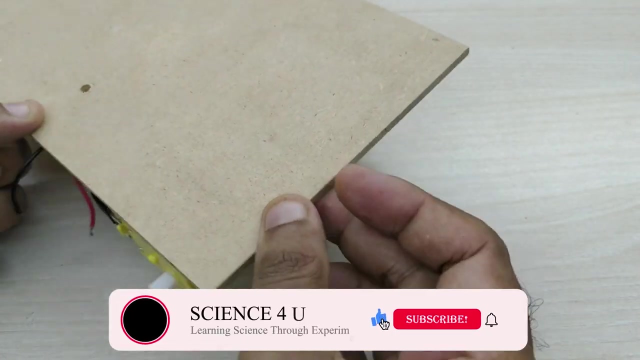 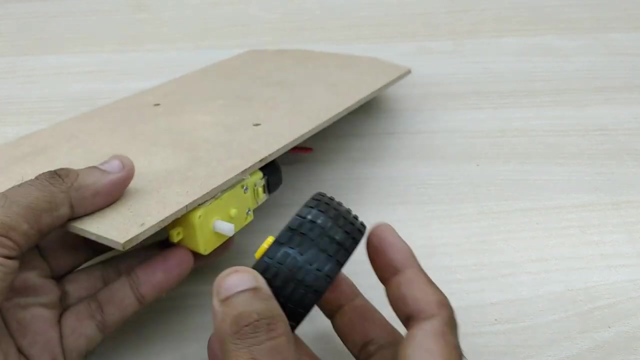 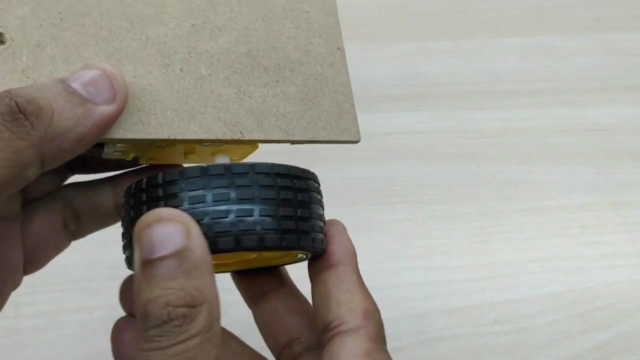 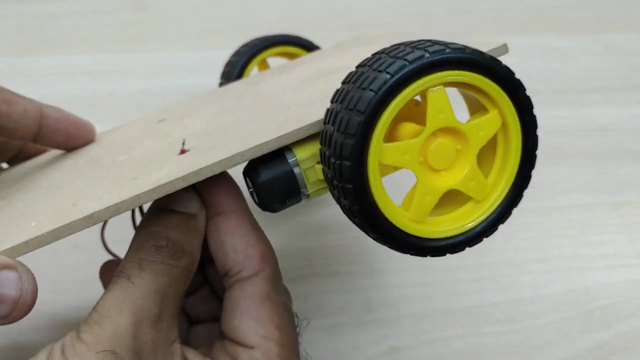 First we have to fix the two motors on either sides, as shown in the video. Our優 Всем. Let us first cut the Arduino miracle wheel, as shown in the video discussions. Now fix the wheels on both the motors. Take the positive and negative wires of both the motors through the hole from below to two. 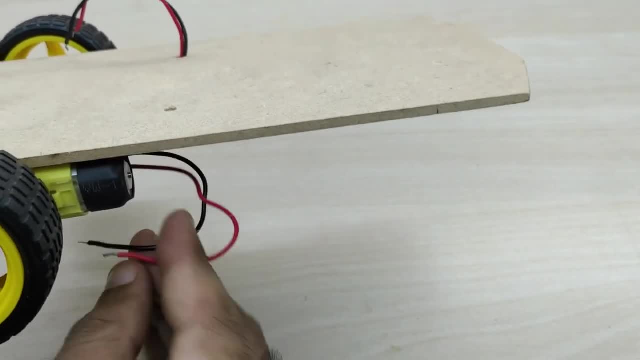 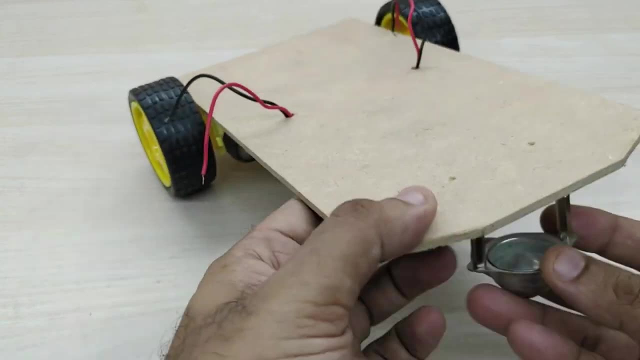 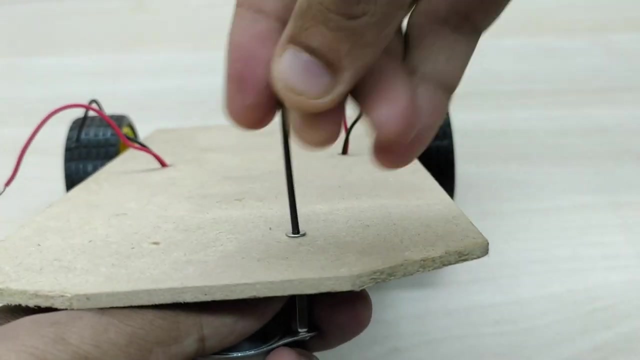 Let us use the scissors attackform. take the positive and negative wires of both the motors through the hole from below to two to the top. Now we have to fix the caster wheel at the front. Providing a caster wheel at the front helps the robot to quickly change direction, since 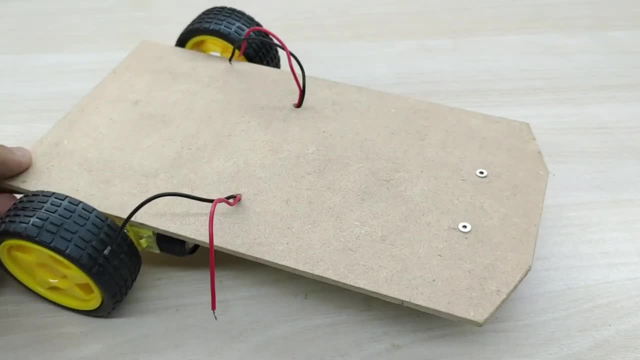 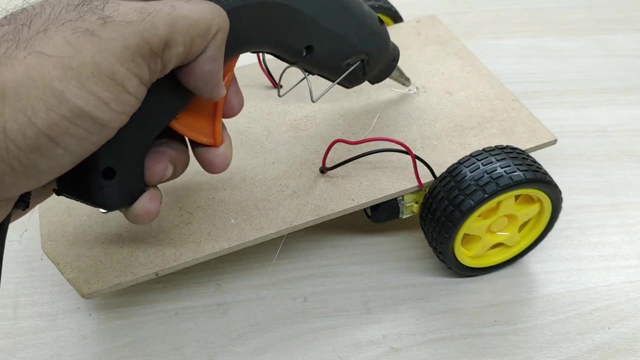 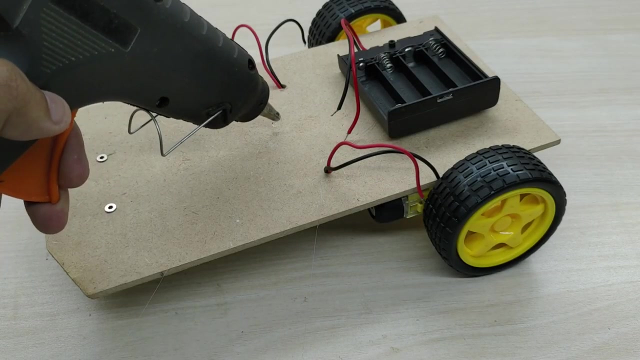 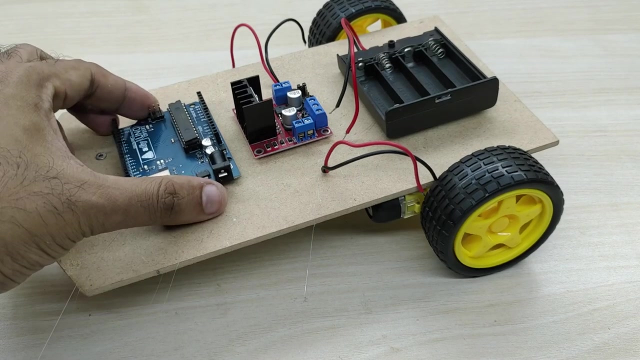 it has a ball that can roll in any direction. Now fix the battery pack, L290A10 motor driver and the Arduino board as shown. Fix the SG90 servo motor module. Now we have to fix the battery pack, L290A10 motor driver and the Arduino board. 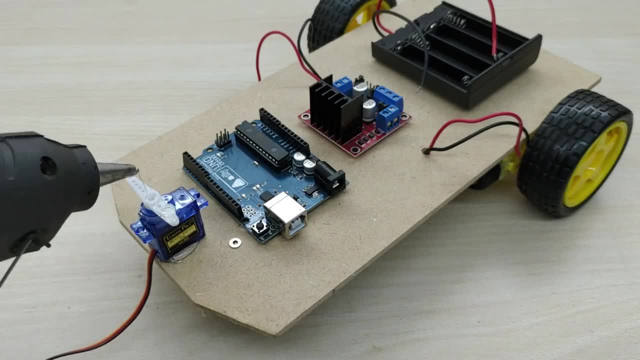 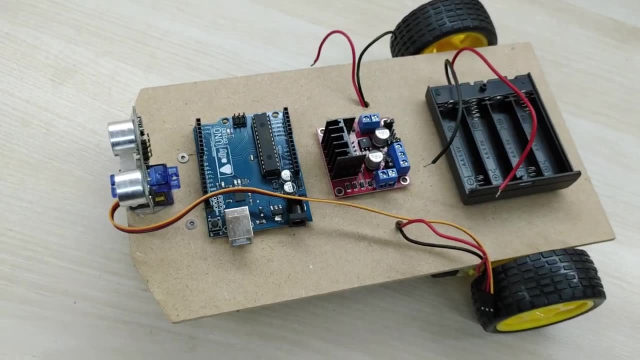 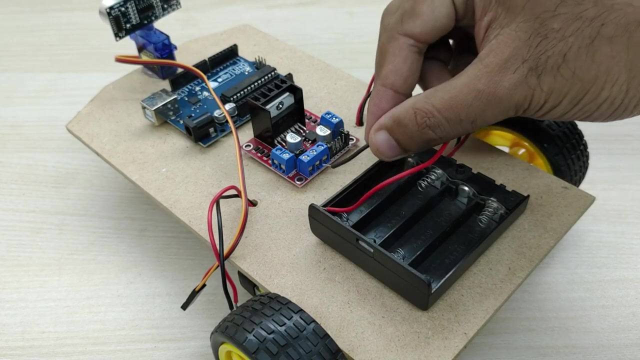 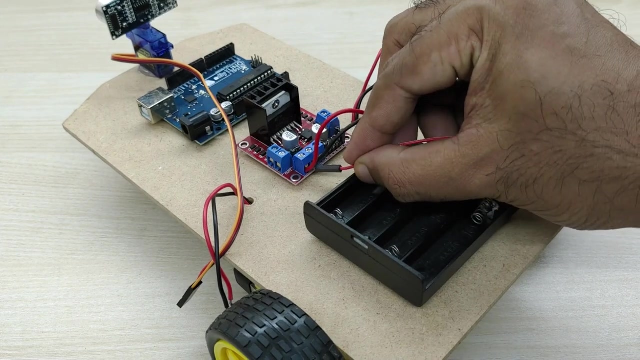 Also fix the ultrasonic sensor on the servo motor module. All the parts are now fixed. It is time to give the electrical connections. First connect the positive terminal from the battery to the positive input terminal of the motor driver board and negative terminal from the battery to the ground terminal of 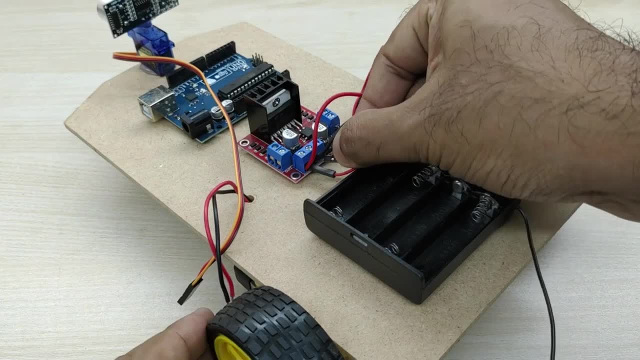 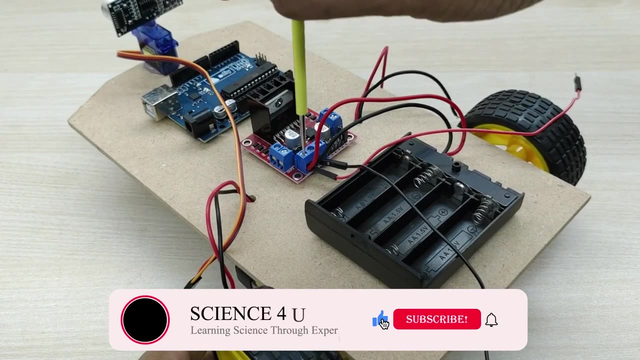 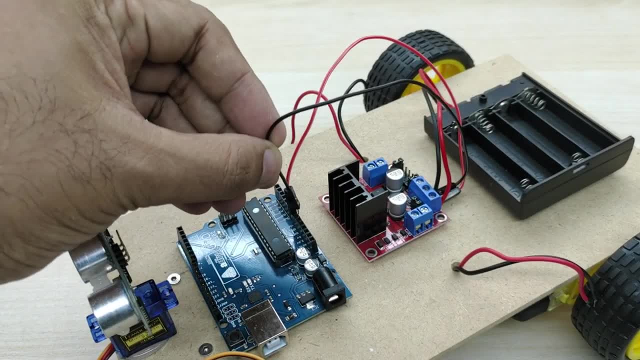 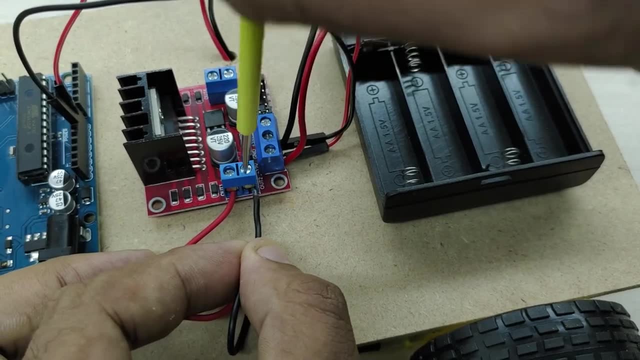 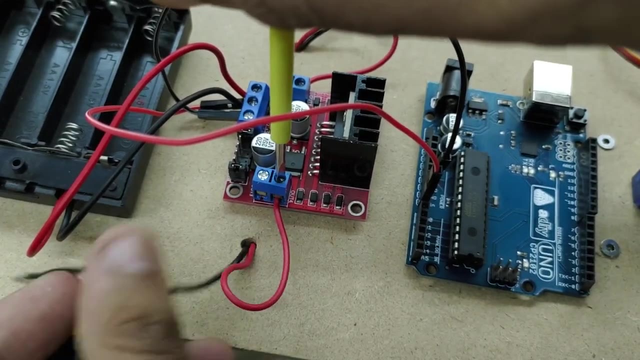 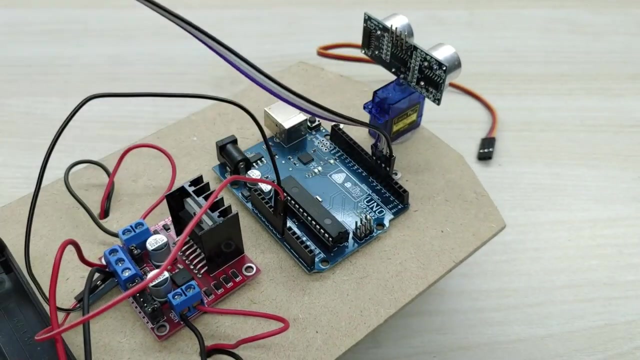 Arduino board. Connect the other jumper wire to ground pin of the Arduino board. Now connect the electrical wires from both the motors to the motor driver module as shown. Take 4 jumper wires and connect them to pin numbers 4, 5, 6 and 7.. 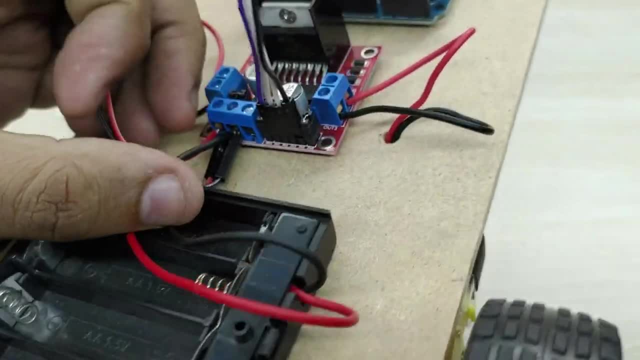 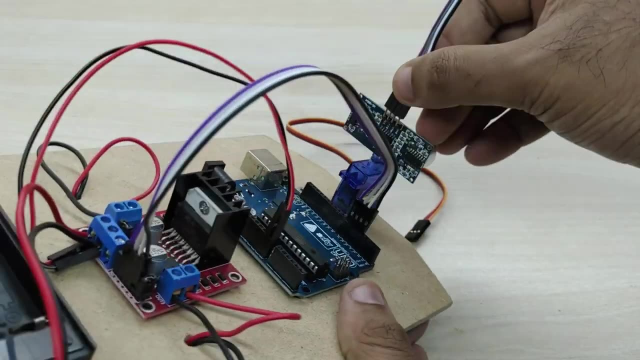 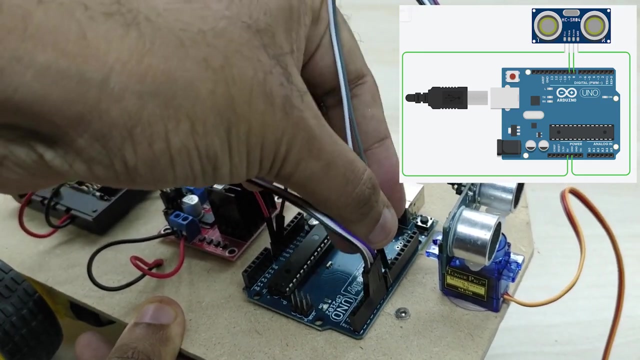 Connect the other end to the motor direction control pins of the motor driver board as shown. Connect another jumper wire to the ultrasonic sensor. Connect the echo pin of the ultrasonic sensor to pin number 8 of the arduino board. trigger pin of the ultrasonic sensor to pin number 9 of the arduino board VCC pin of the sensor. 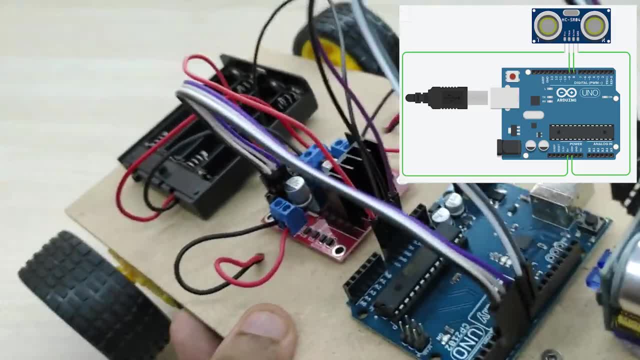 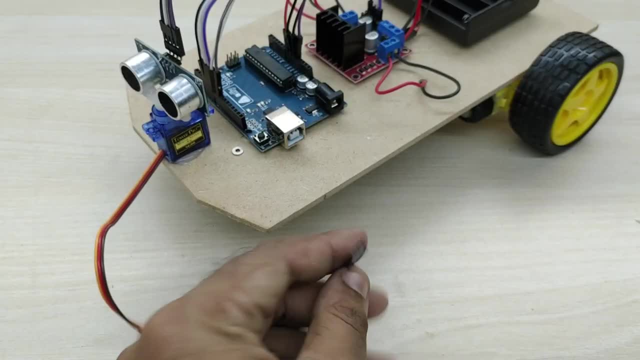 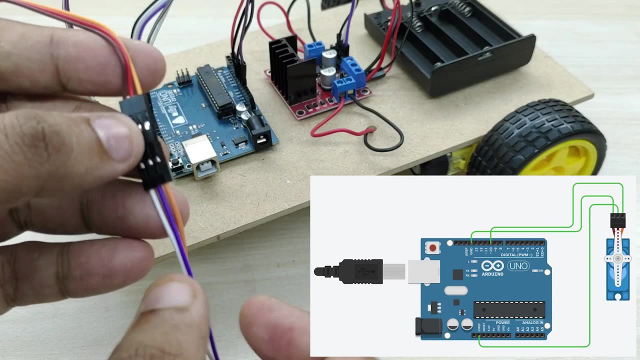 to plus 5 volt pin of the arduino board and ground pin of the arduino sensor to ground pin of the arduino board. Now connect jumper cable to the servo motor. Connect the signal cable, orange wire from the servo motor to pin number. 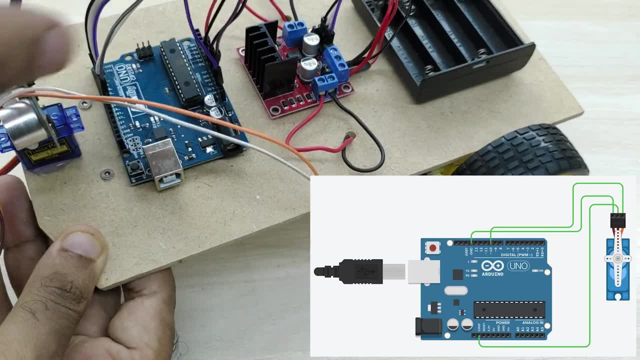 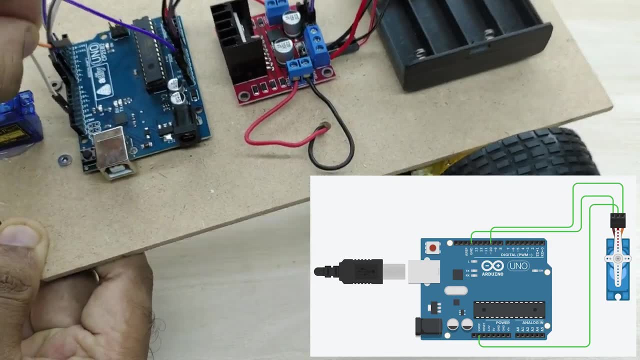 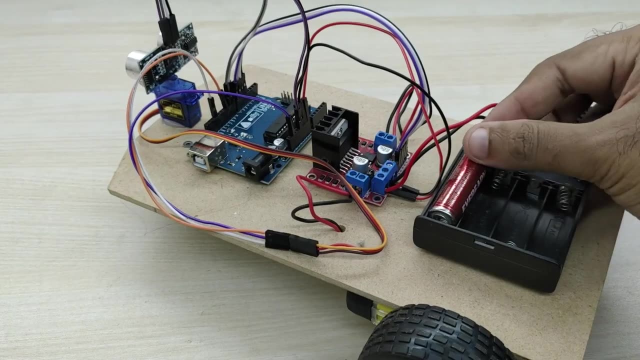 10 of the arduino board. power cable- red wire to plus 5 volt pin of the arduino board and ground cable- black wire to ground pin of the arduino board. The batteries have to be now installed in the battery pack.